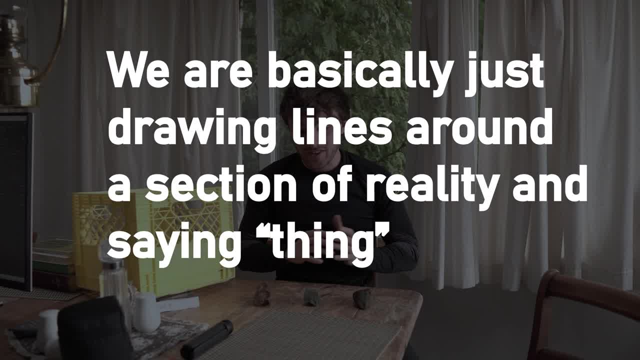 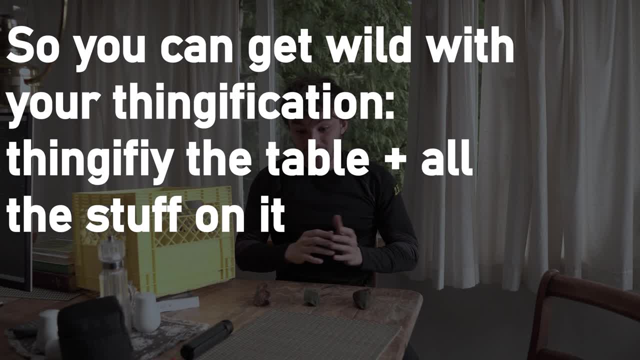 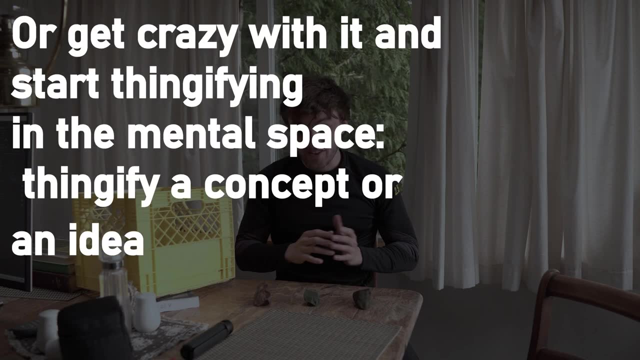 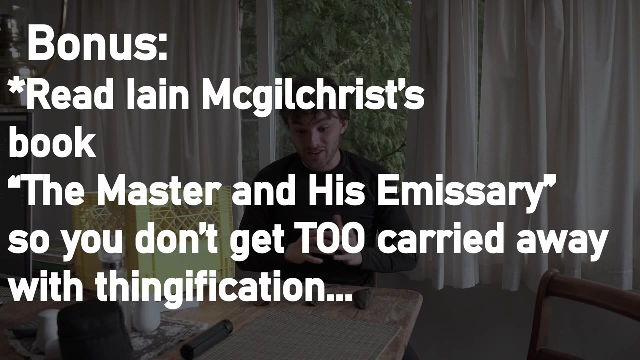 So, one of the things that I wanted to break off of is the notion that you need to identify this foreign variable the emergence of what you need to recognize, because what you've really done now in the day of the earthquake is not trying to tell you— after it had happened, you had to work on it. It was her beginning. Because it was her beginning, it was her ending, which is always her beginning of the story. It's the ending that really set a lot of the our Shocker��서 environment together with the information that you're making out there." Yeah, absolutely. Right. 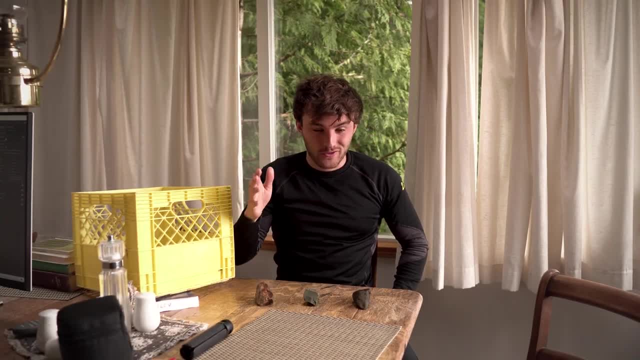 We can talk about the set of all real value functions from the real numbers to the real numbers. 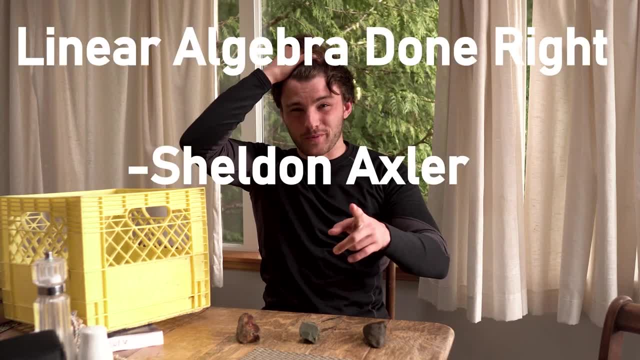 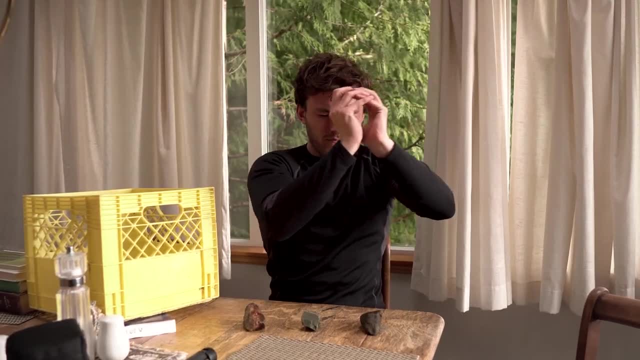 That confused me oh so bad when I was first reading. That was in Linear Algebra Done Right by Sheldon Axler. That confused me for a long time. I started to get it. It's just we're thingifying stuff. Just imagine brackets, got this complicated thing. Shmoop, now it's a thing. 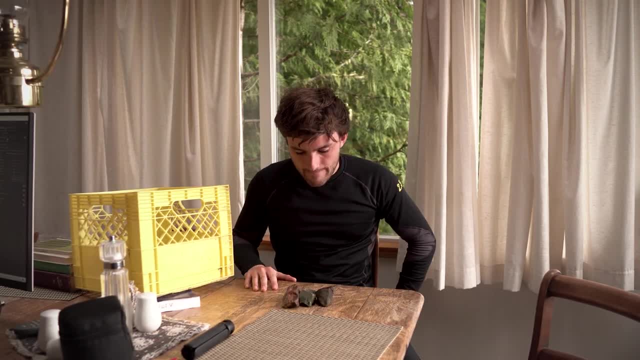 And so we got thing, thing, thing. We put it all in a set. Abstract algebra, the question that abstract algebra is asking, right? So we have this set and we have some stuff in it. 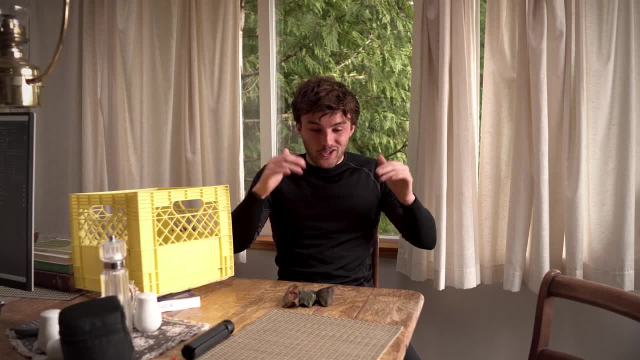 And this is abstract algebra, so it's a little abstract. The problem with abstract algebra, as a side note, it's hard to get a concrete example 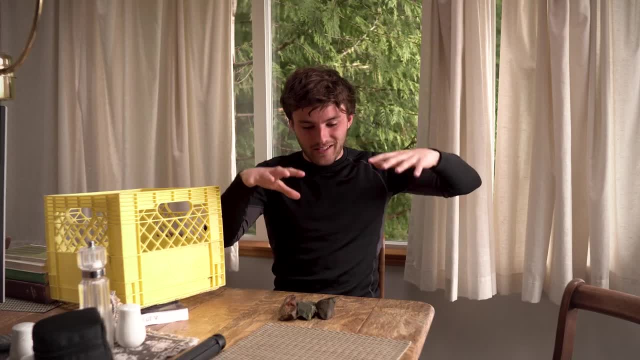 because it is abstract algebra and it was made in the 1800s and it was abstracted from mathematical fields. So it wasn't looking out in the real world and just boop, here's math. 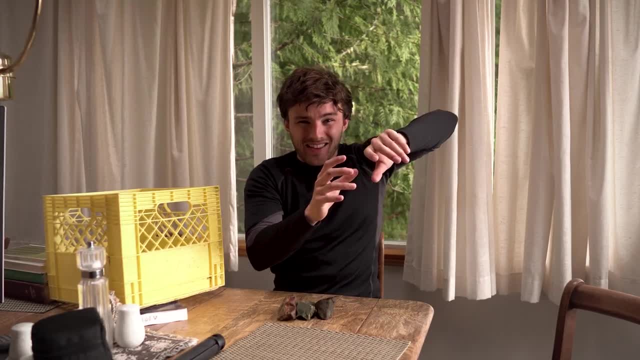 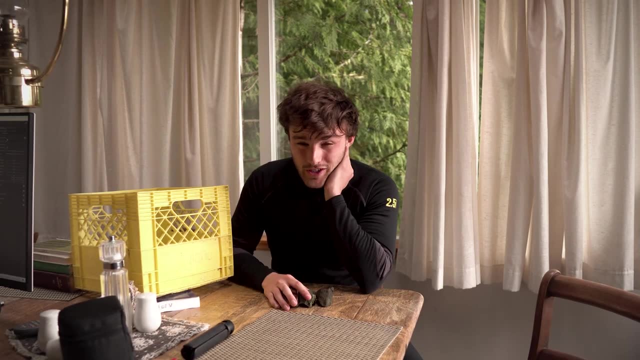 So we have a ton of examples as to where it comes from. It's like, okay, real world, math, abstract algebra. So it makes sense if you have all these maths, but it's also a hard approach. It's just, it kind of came about, it's just tough to have real world examples. So the progression of how it came to be does make sense. It just takes a while of learning mathematical history and stuff. That's still ongoing. 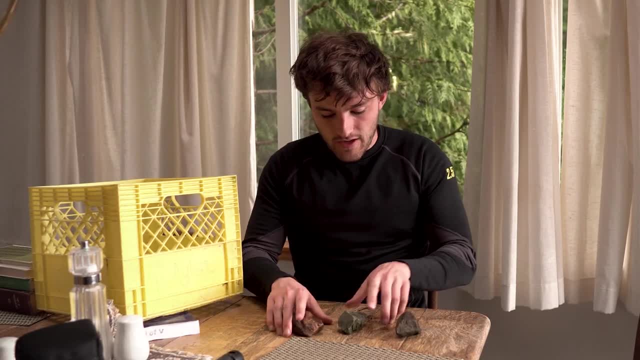 Anyway, the question abstract algebra asks is, you have some stuff. What happens when we take two of these things, shmoof them together? What comes out? That's abstract algebra. 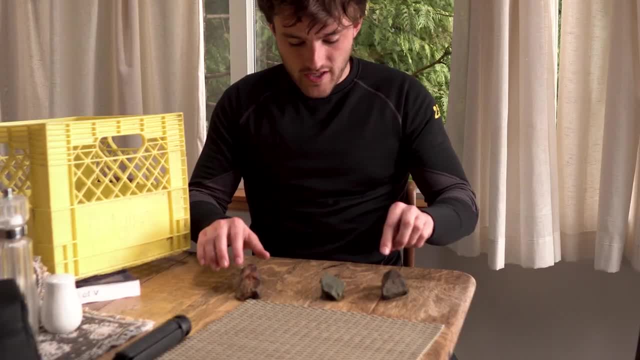 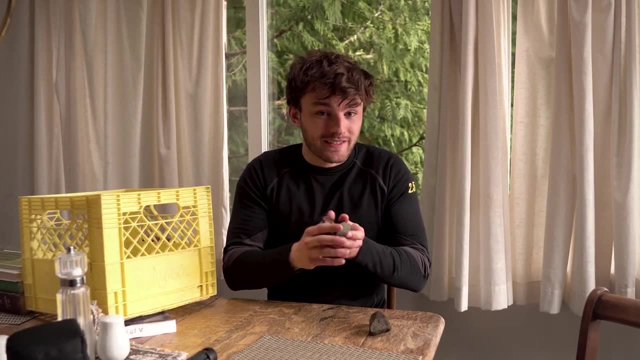 You have some stuff and you say, this is like rock one, rock two, rock three. What happens when we combine rock one and rock two? And pretend these are special rocks. You can like shmoof them together and then another rock comes out, like one rock instead of, it's not like two rocks now. So think of like paints. Paints is another good example. 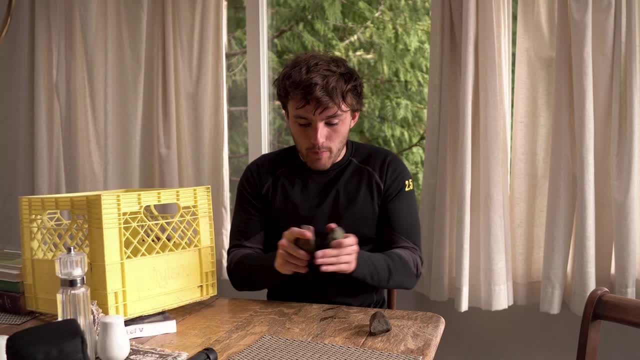 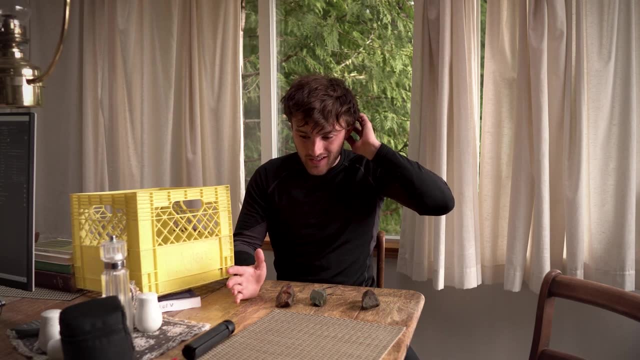 You take two paints, you mix them together, one paint comes out. So you have two things, you put them together, one new thing comes out. Well, not a new thing per se. There is algebra, but this isn't true. But as far as I can tell, and in all the books I've seen, when you combine them together, the thing that comes out needs to also be one of the things. 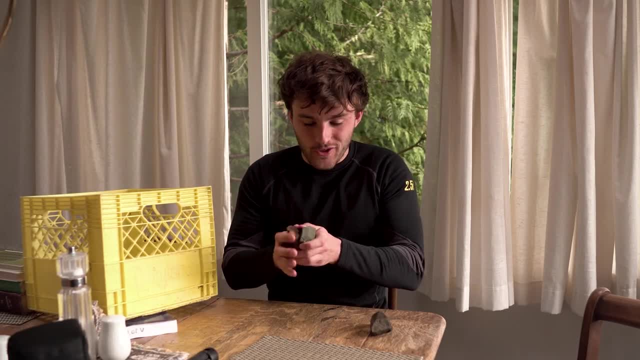 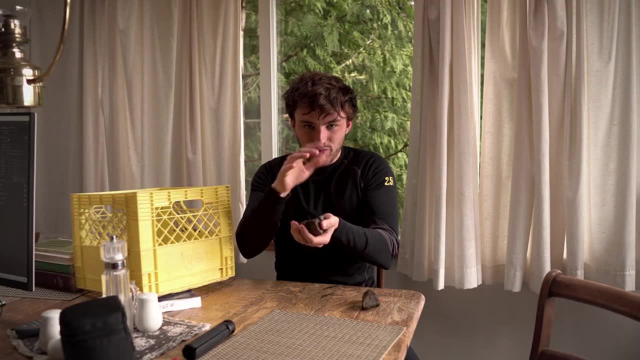 So if you're operating with like a set of rocks and you combine two of the rocks together, the thing that comes out needs to be also one of those rocks. I mean, it could even be this one. Like you combine these two together and then what comes out, just pretend he's like shmoofed together to form one rock. 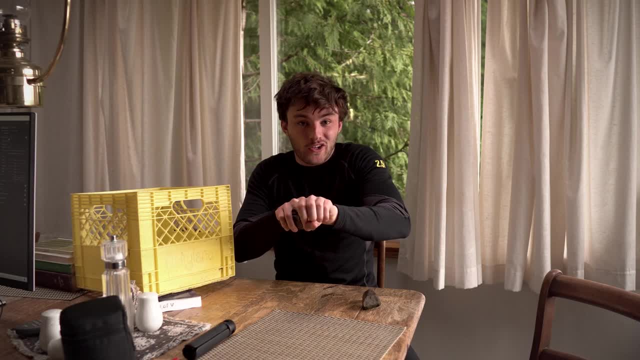 Yeah, it's not the greatest example. But you shmoof them together and then this could be the rock that comes out. 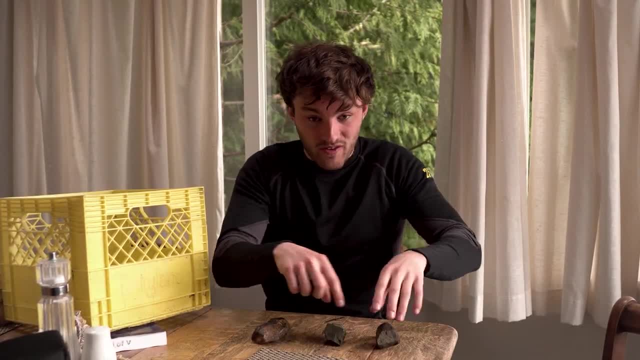 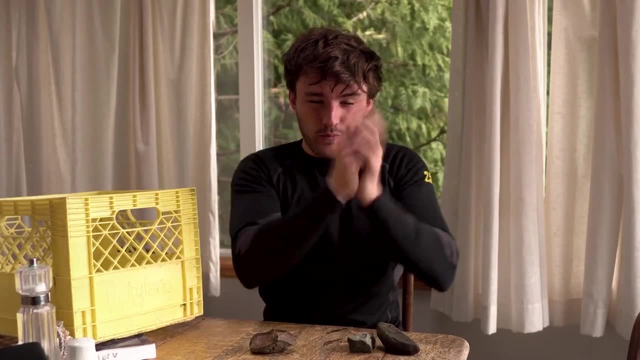 It could just go back to itself. But anyway, it has to be within, it has to be one of the rocks. So you take two, boom, put them together. What comes out? That's the question. You're combining things, items, you're shmoofing together. What's coming out? What color do we want here? Let's go blue. Yeah, I need a black pen. But right now we're working with blue. 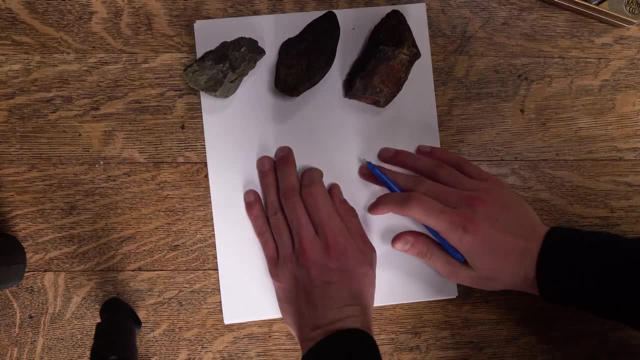 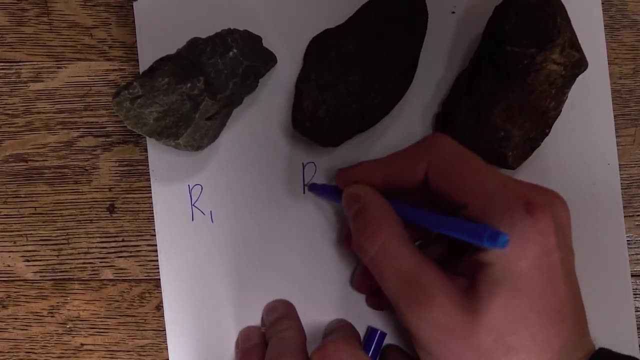 So I'm gonna get annoyed with moving these rocks around. So, and this is a classic, classic mathematical thing to do. We are just gonna call this rock, rock one, rock two, rock three. 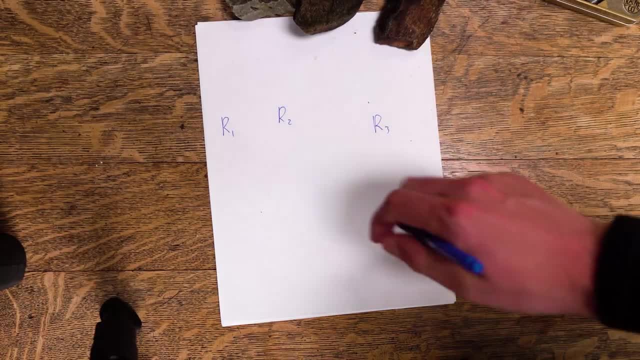 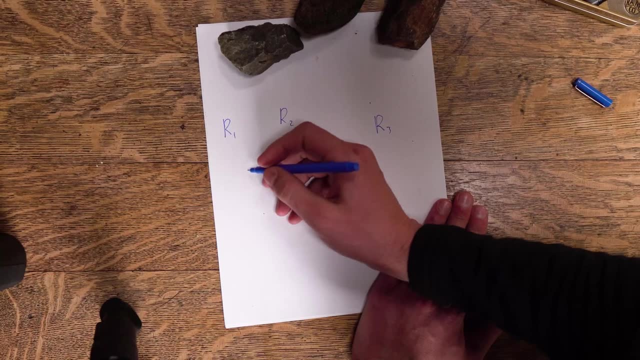 And then we can just get rid of these. I'll leave these at the top of the screen. We wanna see what happens, right? The shmooping. We wanna see what's going on with the shmooping. So we're gonna go ahead and create a table. We're just doing, we're just getting quirky. You know, we're just gonna quirk them out. We're just like, you know, we're like, all right, let's just see what's going on. Let's just see what's happening. So we're gonna go ahead and create a table, right? Cause we wanna see what happens 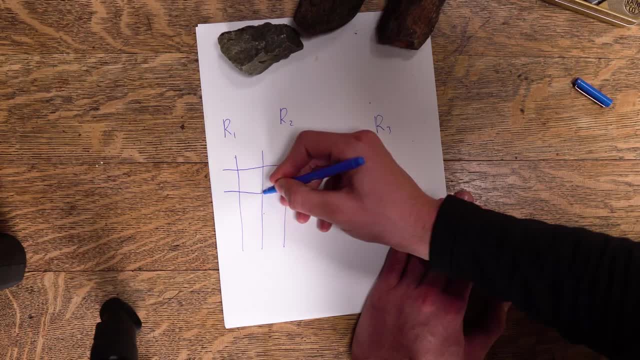 when we combine the rocks together. And also order matters. So we're gonna have to do every possible combination. So, you know, R1 combined with R2 might be different than R2 combined with R1. You know, this is just, we're getting quirky. 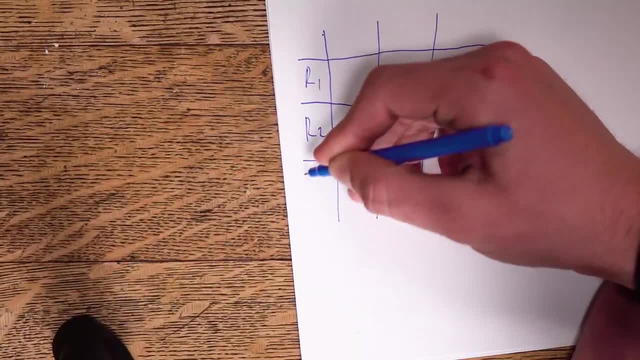 We're just getting crazy. And so we're gonna go R1, R2, R3, R1. 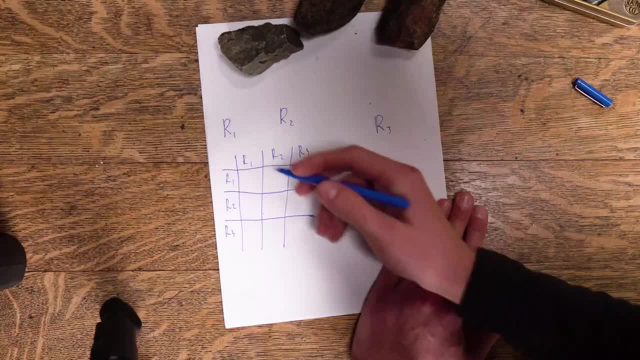 We're just coming up with a table. We're just trying to come up with some way to represent what happens when we combine all these items, right? 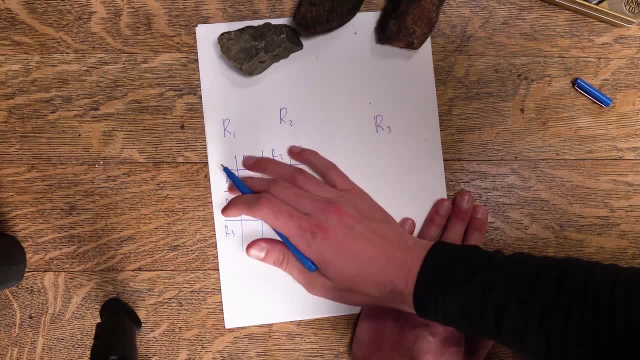 Okay, and so in these, this is just like, what happens when you go R1 combined with R2? I think of it like, because order does matter, unfortunately, so it's not as simple. 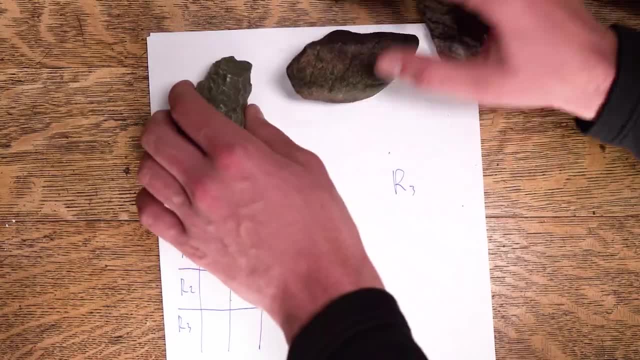 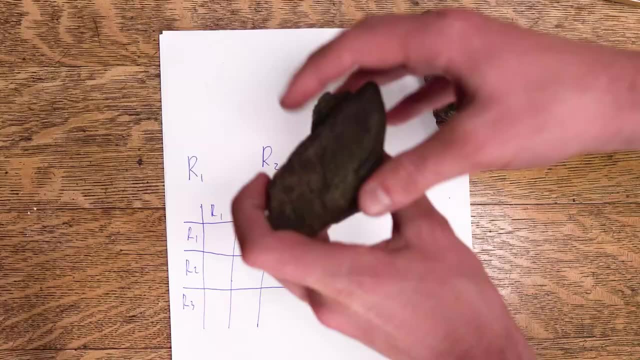 What you're gonna do is think like R1 combined with R2. I think this is R1, right? It's like on top. And then I think of R2 combined with R1, like it's on top. So they might be different things. Sometimes they're not. Sometimes they just, they're like paint and it doesn't matter what order you put them in, but sometimes it's gonna matter if it's R1 on top or R2 on top, it'll matter. 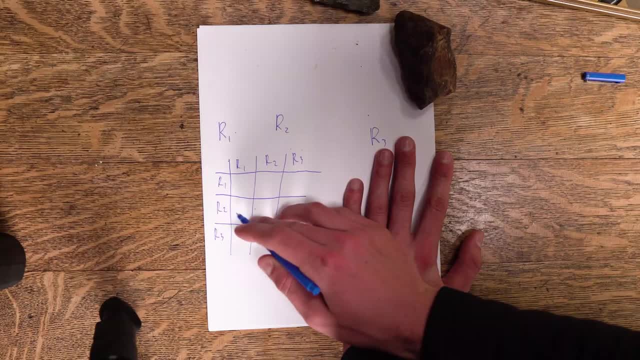 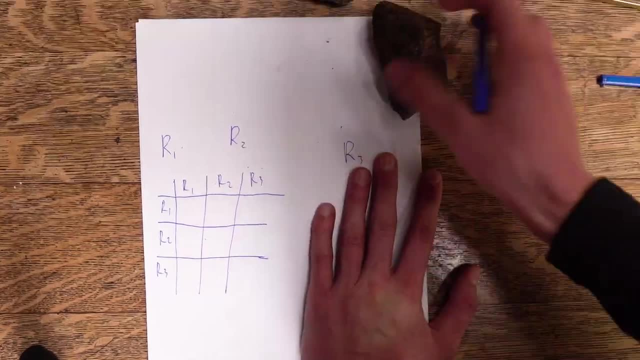 And so now we have every possible combination. So this is like, this box right here means R2 on top, R1, what happens there. And we can fill this in however we want, really, here. So I'm just gonna arbitrarily fill it in. But the only rules are, they need to be, the things in these boxes need to be one of the R1, R2, R3. So I'll fast forward this. Hey there, Future Tucker here. 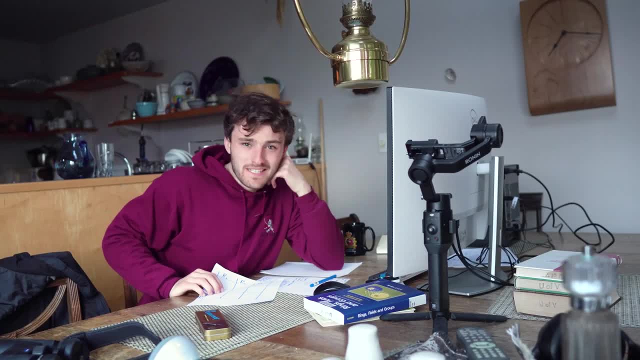 Just a quick interjection. As I was editing this video, I realized it might be a little confusing with the notation, so I just wanted to go over it a little bit better. 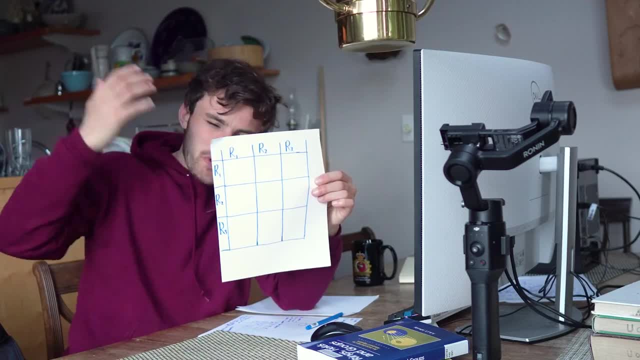 So with this chart, what we're doing, really, at the end of the day is we are combining elements, right, of a set. We're taking things and we're schmooping together and we're seeing what comes out. 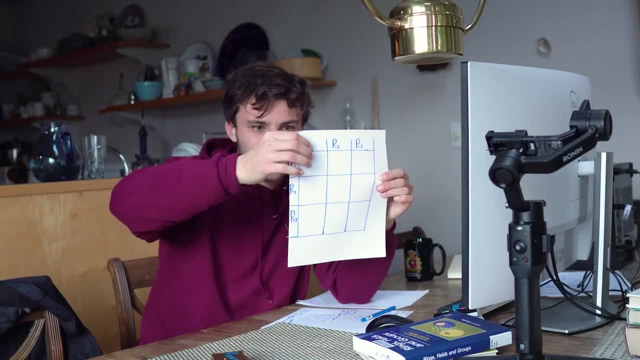 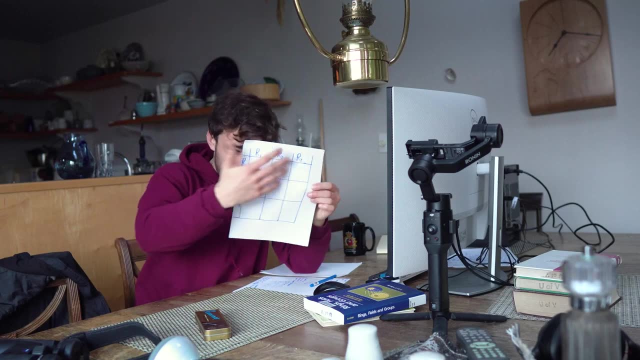 And we want a visual way to represent every possible combination of the combination of things. Every possible schmooping, we wanna have some way to write that down. And so we just, we're like, hmm. We ponder, we think, we contemplate, and we come up with this thing. It's just a way of representing every possible schmooping and writing it down. 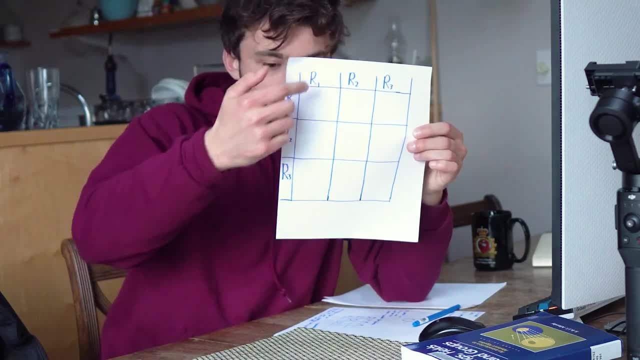 So this box is gonna be R3 combined with R1. When you take R3 and combine it with R1, that goes here. 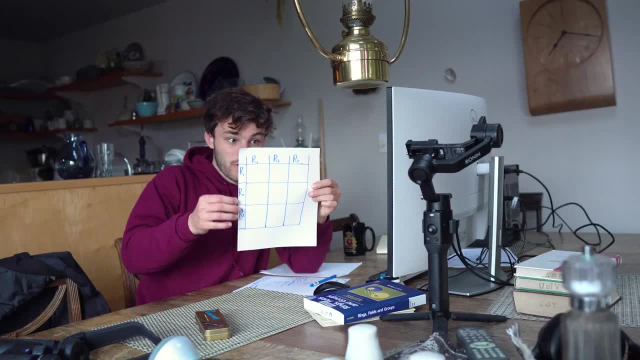 Or you take R3 and you put it on top of R1, that is what comes out here. And then over here, this is what happens when you take R1 and put it on top of R3 and schmoop together. So order does matter. It's unfortunate. That's why concrete examples are really difficult because it gets very hairy. 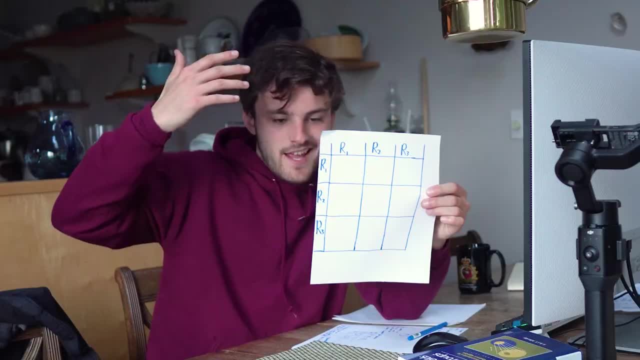 But the idea is there. The way I think about it is as if you were a scientist and you're combining stuff in a lab. 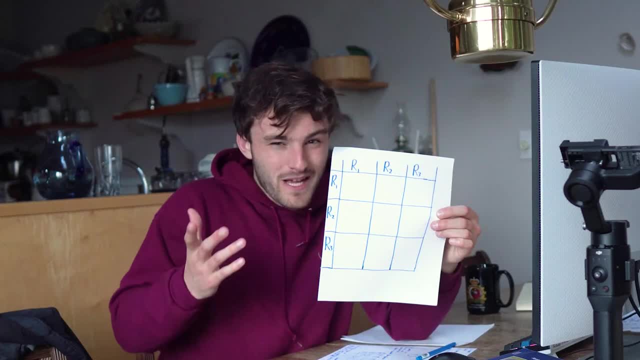 Say it's like chemicals or, I don't know, rocks. Let's pretend there's rocks. And there's special magic rocks, so they do some stuff. 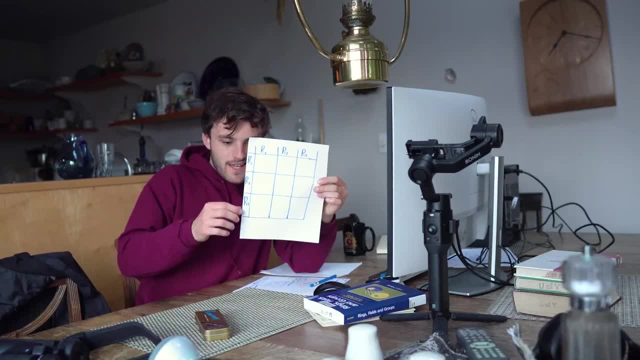 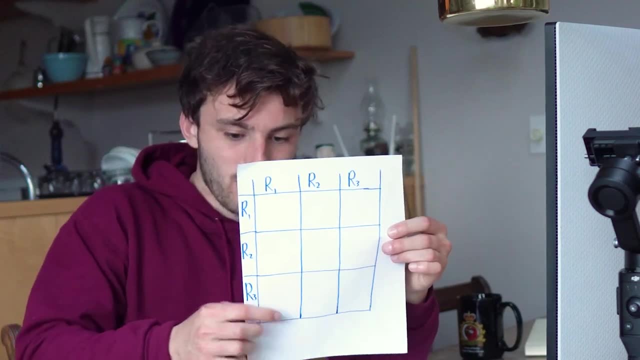 And so you're experimenting. You have these rocks laid out. You wanna see what happens when you combine them. And then you wanna come up with a way of recording what happens when they do, because you're a scientist. So this is the chart you come up with. When you take R3, you put it on top of R1 and what pops out? You put that thing here. 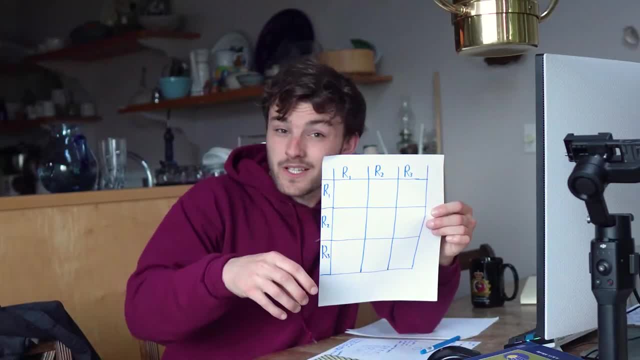 And you get R2 and you put it on top of R1 and you schmoop them together 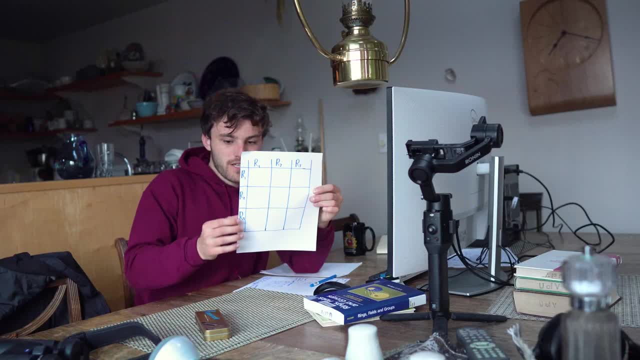 and then there's special rocks. Remember, so they pop out another rock, one rock. That goes here. 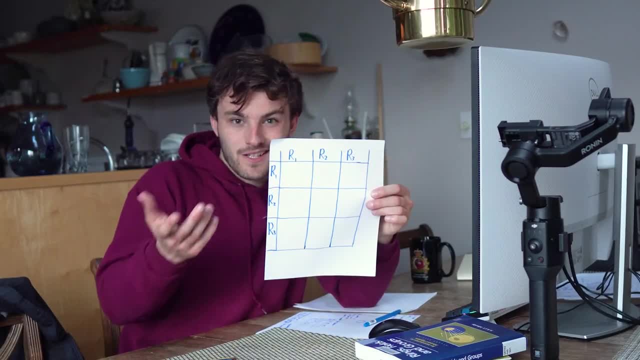 You take R2 and you put it with another R2 because you're allowed to do that because these are, I don't know. The rocks, the rock example kind of falls apart at some point. But you get the idea. You take R2, you combine it with R2, put R2 on top of R2. 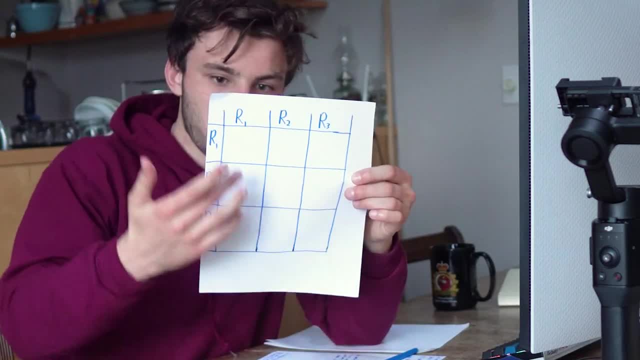 That goes here. You take R3, you put it on top of R3. That goes here, et cetera, et cetera. You can fill this in. You just have to combine every possible combination in every order. 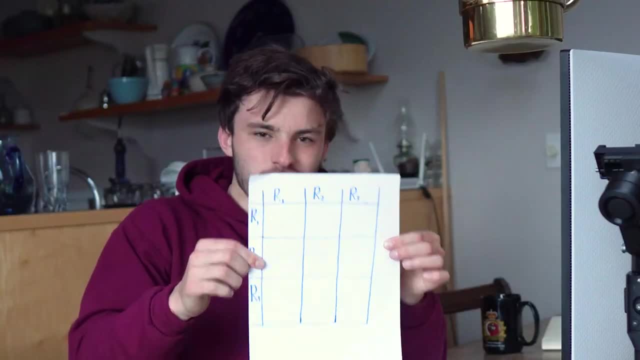 That fills out this whole thing. So this is just a way of representing every possible combination of the elements of what you're dealing with. 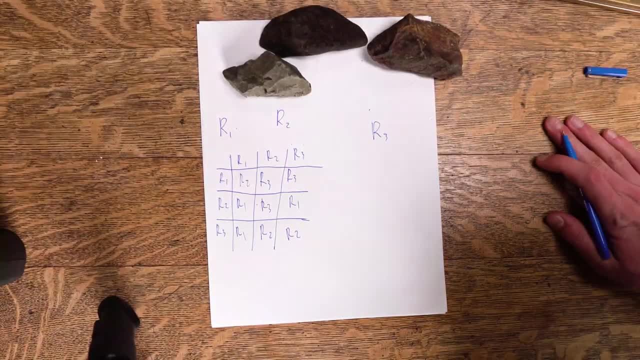 All right, back to the video. And so there you go. I mean, create your own here. 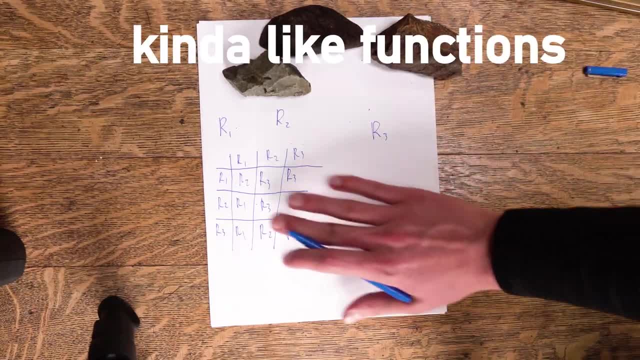 You know, you can make them literally whatever you want. But this is what an al, this is, so if someone says, what is an algebra? This is an algebra. 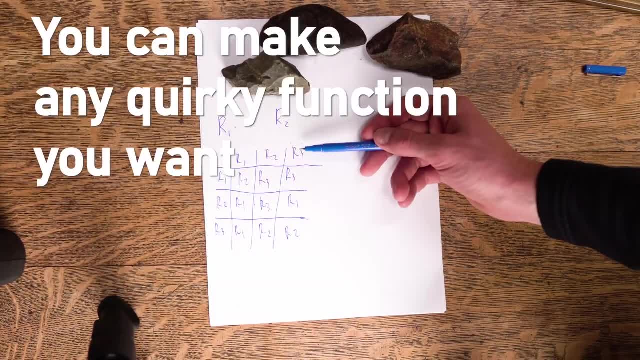 These can be infinitely long. They can be, the set of all people in the country of Zimbabwe. 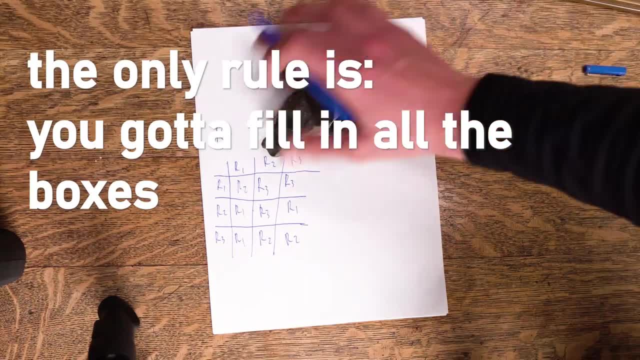 But we're just questioning, you have some items in a set, you have some things, right? Things in a set. And the question is, 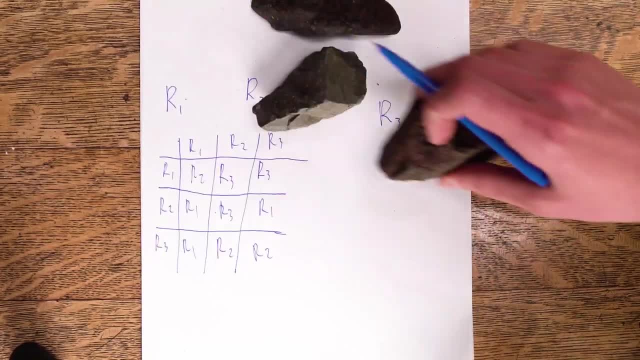 what happens when we combine those things, right? What's going on? We take two of these things and we combine them together. 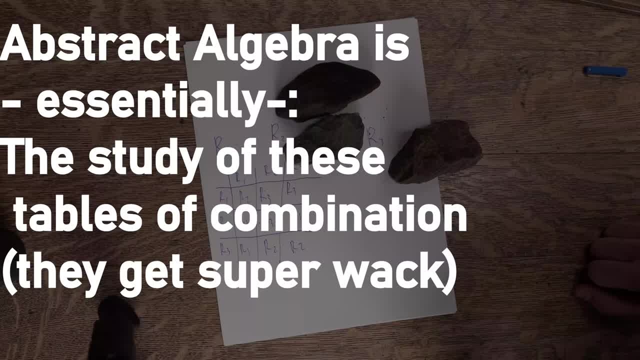 What pops out? Abstract algebra. Okay, now I wanna go on for about an hour cause there's like so much stuff I'm missing. But I gotta make these short, so that's gonna be it. 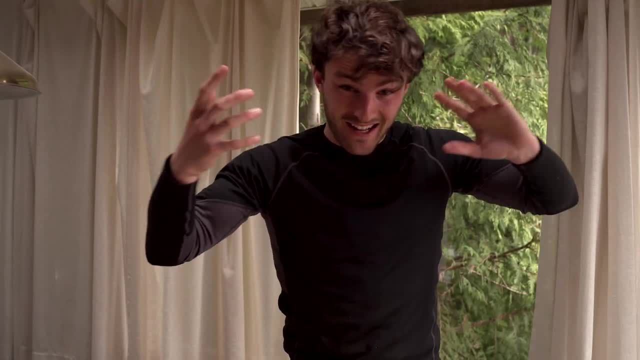 But groups, if you're wondering what groups are, a special case of that. You have some items, how do they combine? But there's some particular rules on how you can combine them. 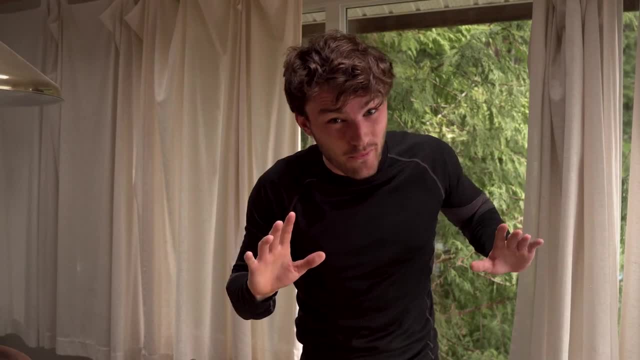 Rings are, you get two different operations and I can't really define rings that well cause I'm still kind of learning what's going on there. 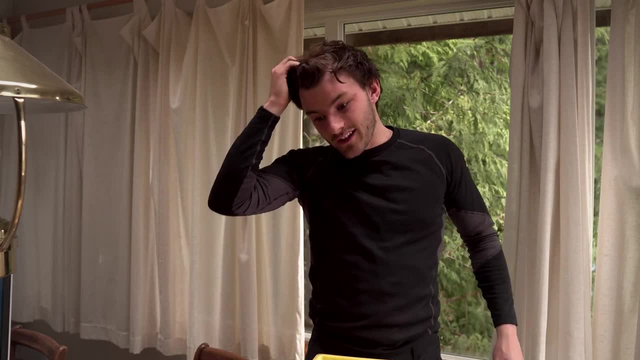 But I'm pretty sure you take two different ways of combining them. And they'll go over how to, there's a way of writing the combination. 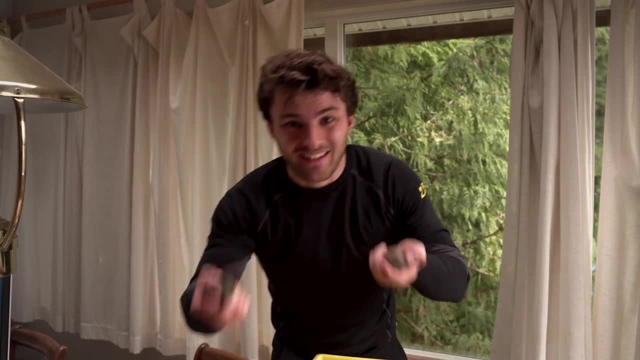 So when you write R1 and R2, you go, I don't wanna have to like, I don't wanna have to take two rocks and go like, hey, when I combine this rock with this rock, what happens? So there's a symbol for how we combine them. 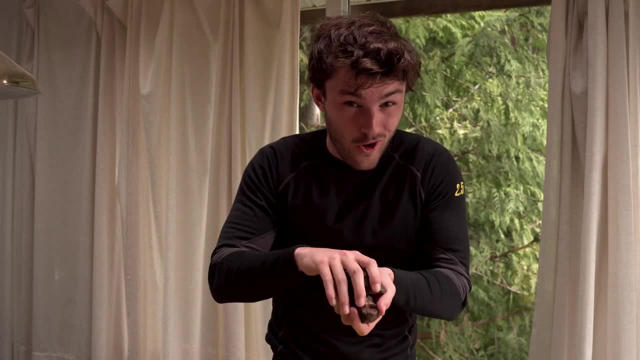 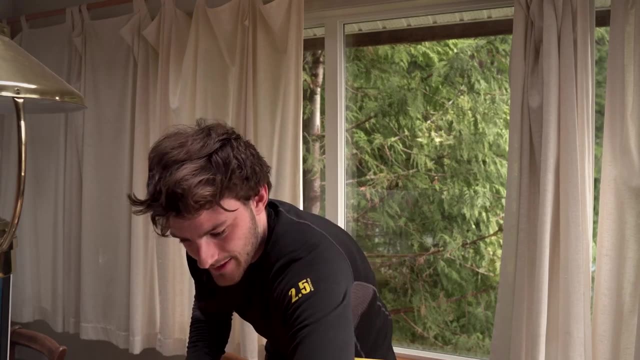 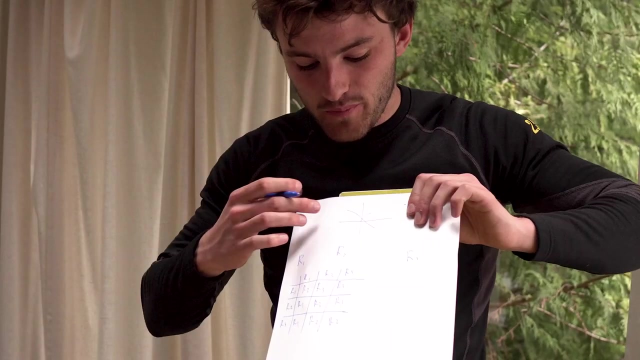 So you have to come up with some sort of symbol to write down like rock one combined with a rock two. And that symbol, you can come up with arbitrarily ones. You can come up with whatever symbol you want really to say like R1 with R2, but damn it. A lot of the time in textbooks, it's gonna be that like star. It's gonna be that puppy right there. And this just means you just put like something here and something here. 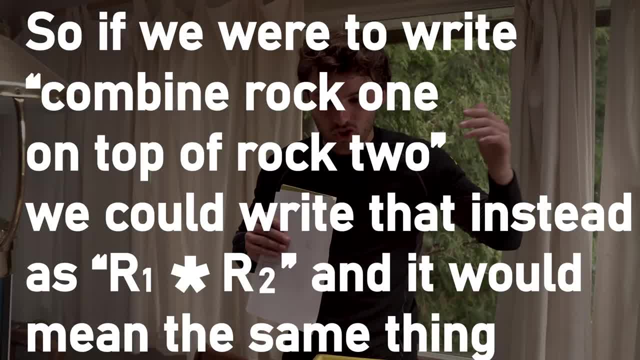 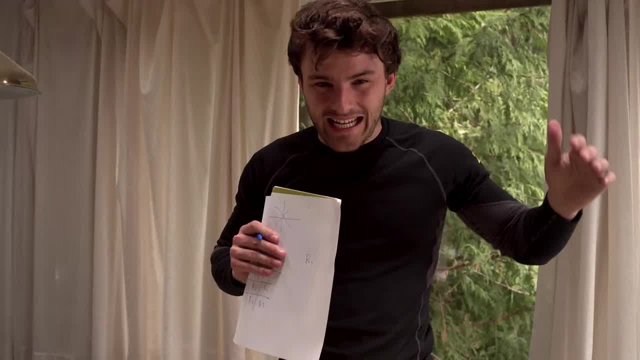 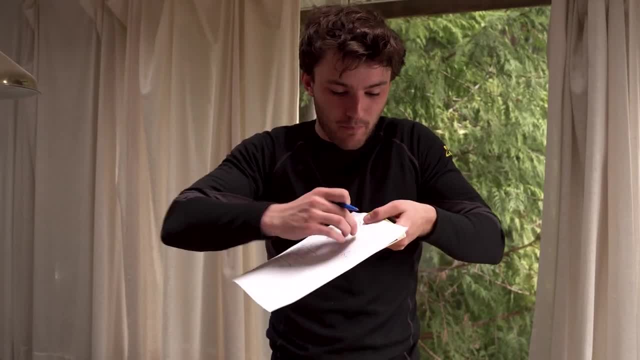 And this symbol, you read it as R1 composed with R2. Or Jack composed with Jill. Or Bob composed with the concept of time. Literally just thingify things and then this is the composition. You put them together and poof, it comes out. Order matters and oh, and also, okay, this is gonna take a while to edit. Still, when you're drawing in algebra, you put the symbol for how they combine right here. 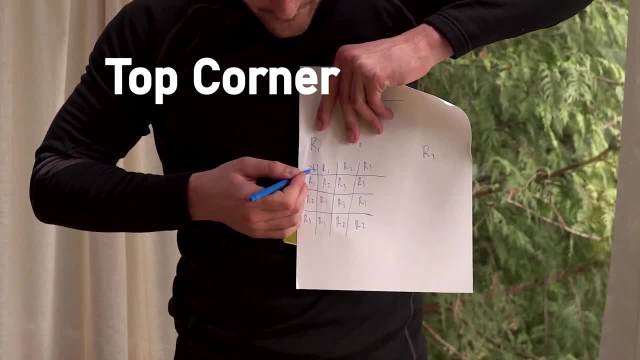 So you just put, this is the thing you put in between two items when you're combining them and you just put it up here just for notational sake. 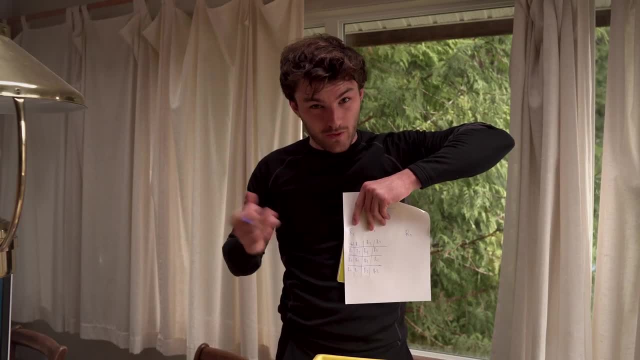 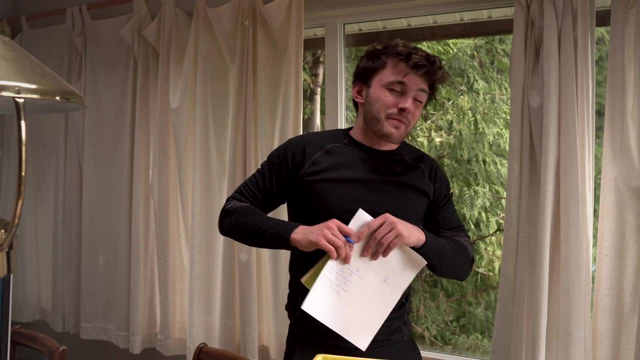 I'm just gonna be a little janky, just kind of stream of consciousness, what's going on in abstract algebra right now for me. And without further ado, that's gonna wrap it up for this episode of Autodidact teaches stuff. 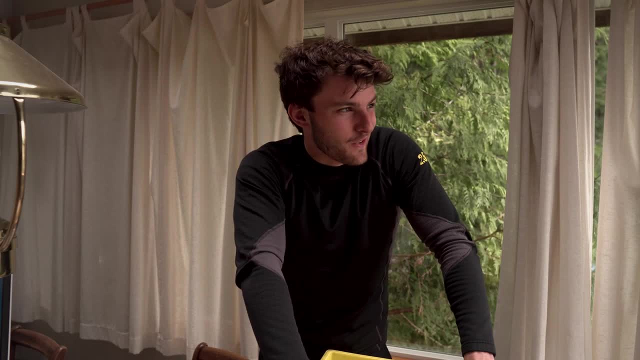 This episode of Pondering with Autodidact. Oh, what else do I call this? Episode of Abstract Algebra in the Woods. 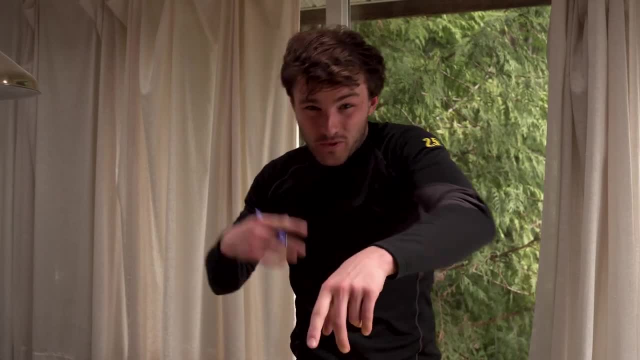 Yeah, that's gonna conclude this episode of Abstract Algebra in the Woods. 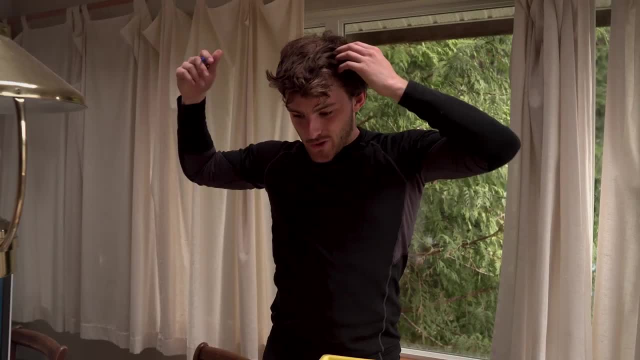 I have been your host, Autodidact. If you liked the video, please subscribe. 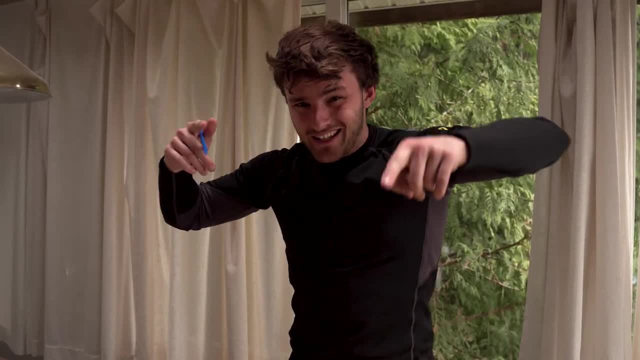 Turn on the post notifications, I'm supposed to say that. And without further ado, take it easy.